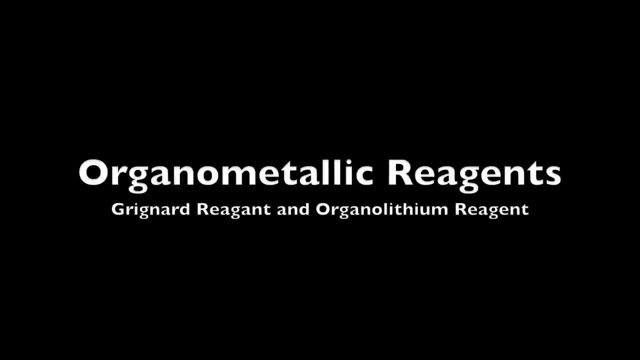 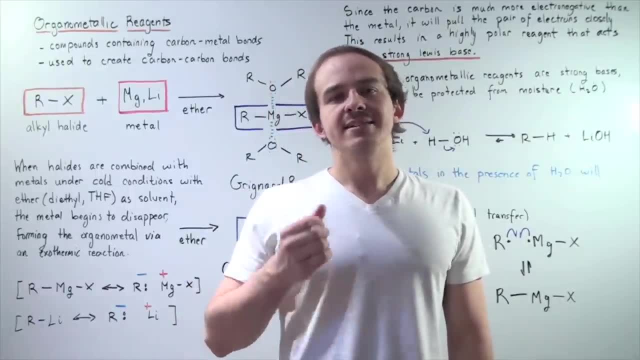 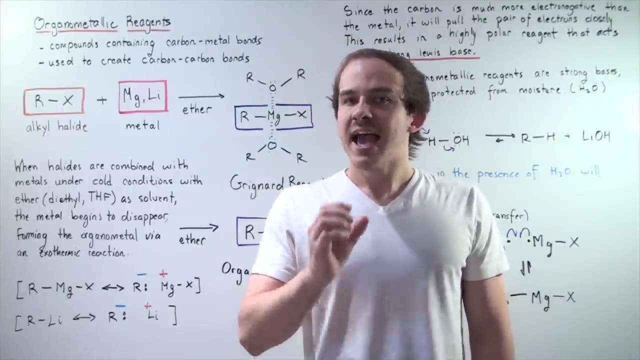 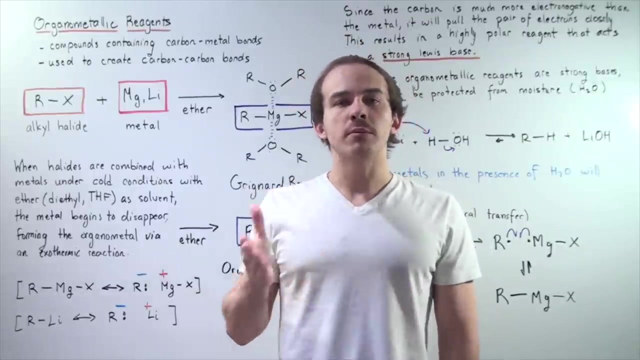 In this lecture, I will give an introduction to organometallic reagents. So what exactly is an organometallic reagent? Well, an organometallic reagent is, simply put, a compound that contains a carbon metal bond, And these organometallic reagents are used to produce carbon-carbon bonds, or carbon-H bonds. In this lecture, we're only going to focus on carbon-H bonds. 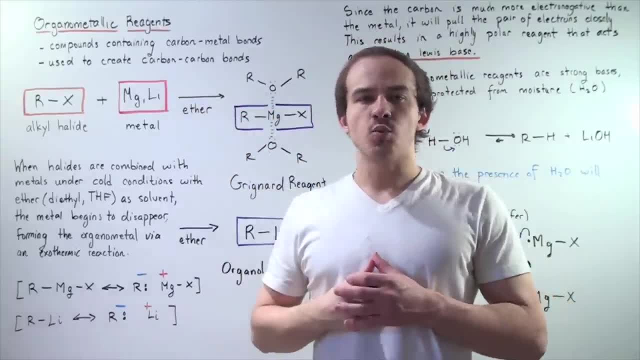 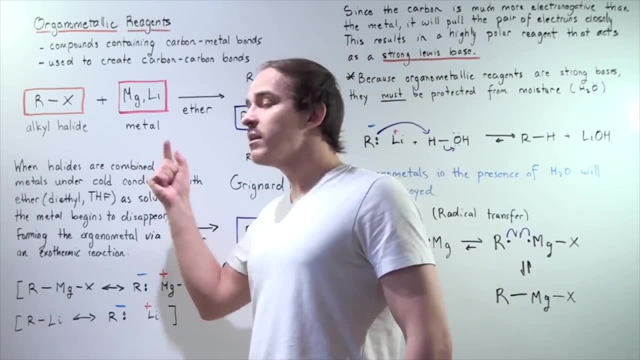 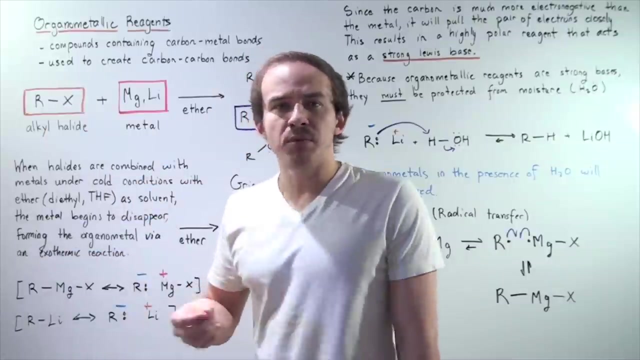 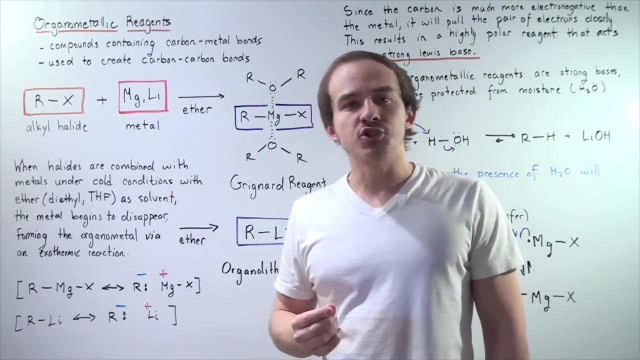 So how exactly does one produce our organometallic reagent? Well, two things must be mixed, two compounds, A metal must be used- either magnesium or lithium- and an alkyl halide. Now, this R group is simply your hydrocarbon group, And that means the carbon is attached to our X, which is simply a halogen. 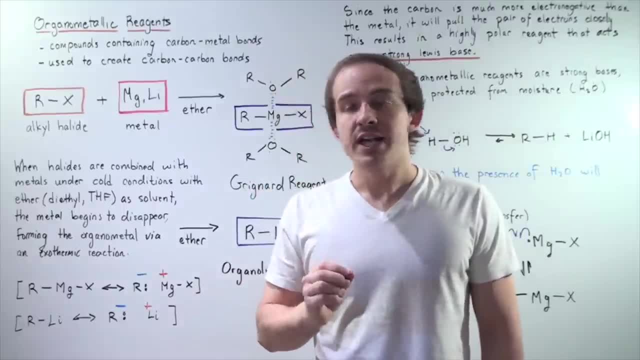 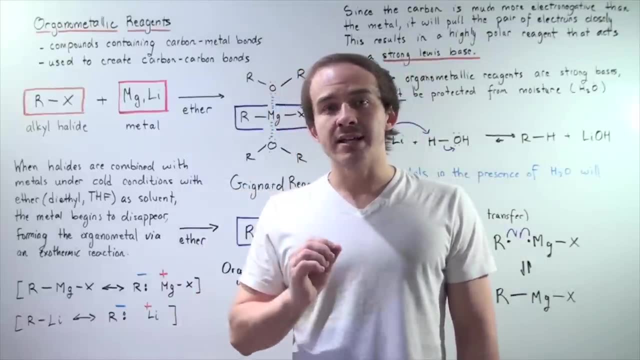 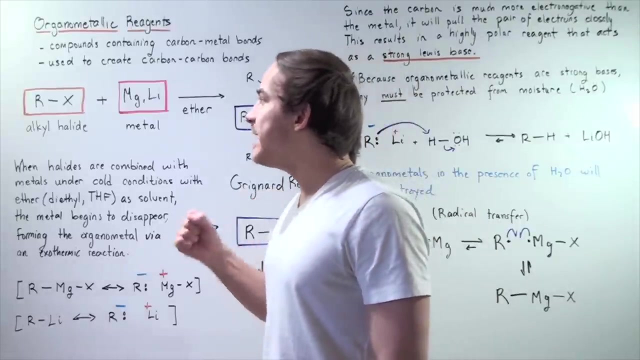 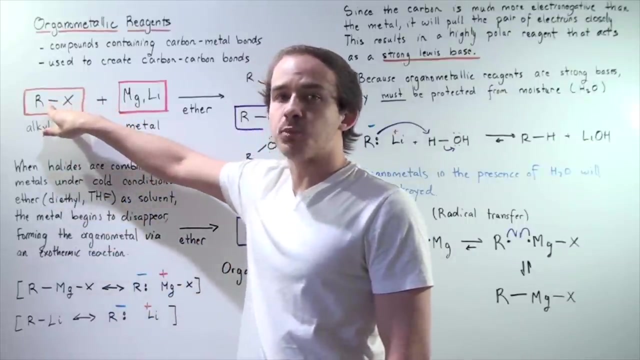 Now it's important for the X not to be fluorine. So the X can either be fluorine or fluorine. It can be chlorine, bromine or iodine. That's because fluorine is very electronegative and it binds very tightly. It creates very strong bonds with carbon atoms. So that means if we use fluorine this reaction won't readily take place because this bond will not break. 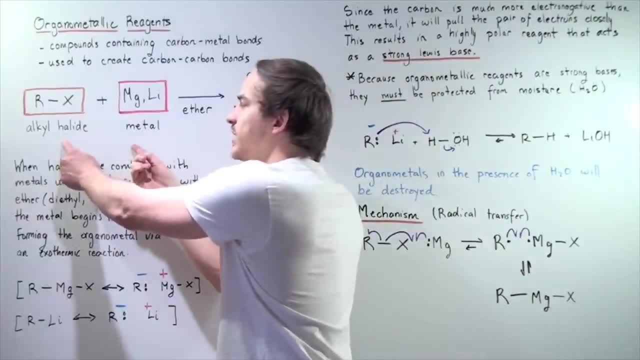 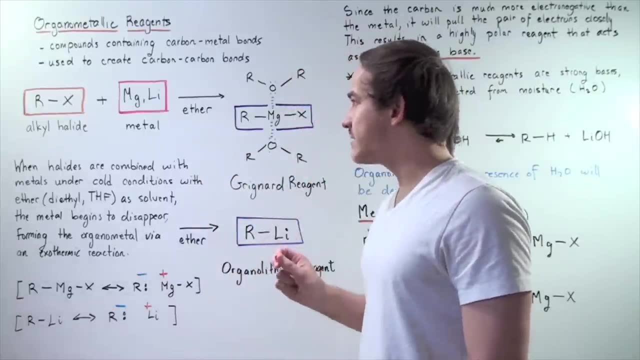 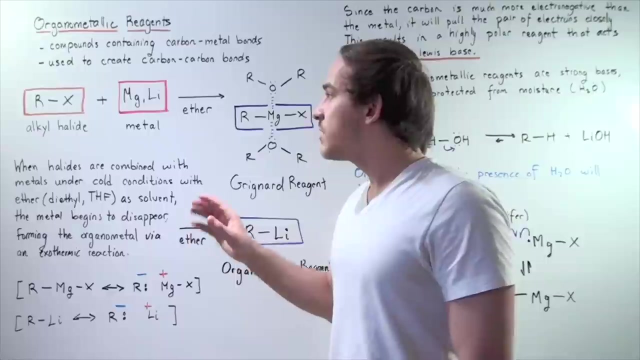 Now, when we combine these two reagents, these two compounds in a solvent, the solvent must be ether. Ether stands for carbon. It stabilizes the product. Later we'll see that if we use a polar solvent such as water, the organometallic reagent will break, It will dissociate, And we'll see why later. 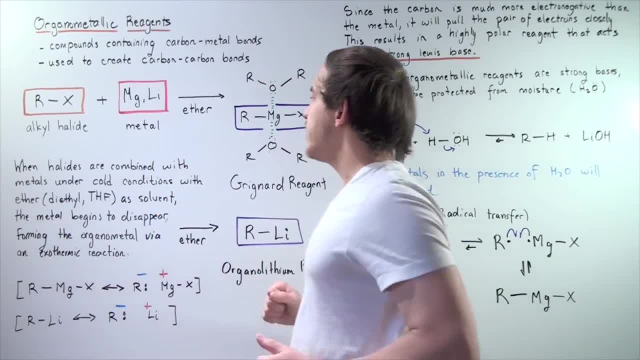 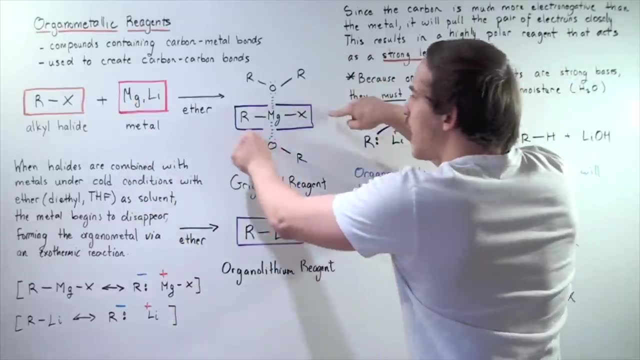 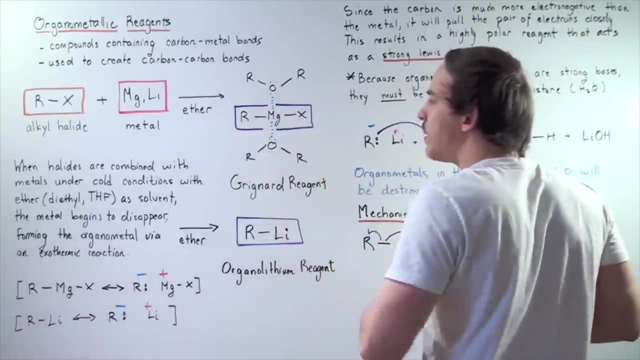 So when these two reagents are used, we produce the following two compounds. So if magnesium is used, the following organometallic reagent is produced, boxed in purple, And so we have the R group, The carbon-Mg bond. 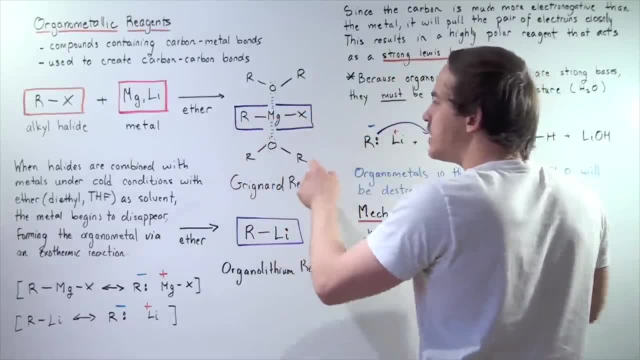 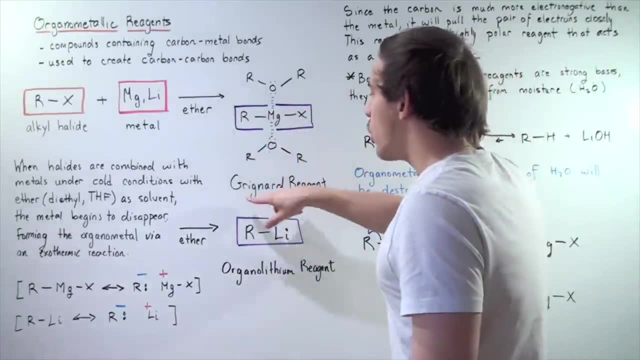 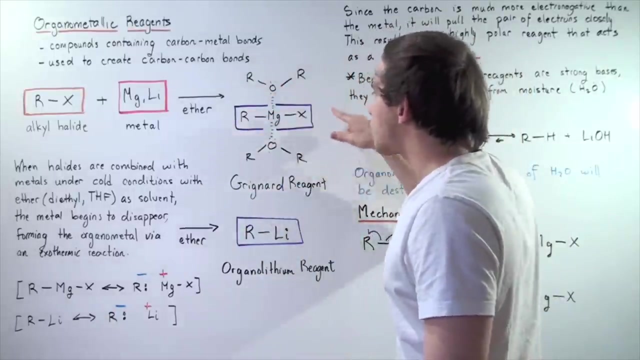 So this is our carbon-metal bond And this Mg also binds to our halogen. So we have the following organometallic reagent, known as Grignard reagent. Now notice that the ether stabilizes our organometallic reagent. 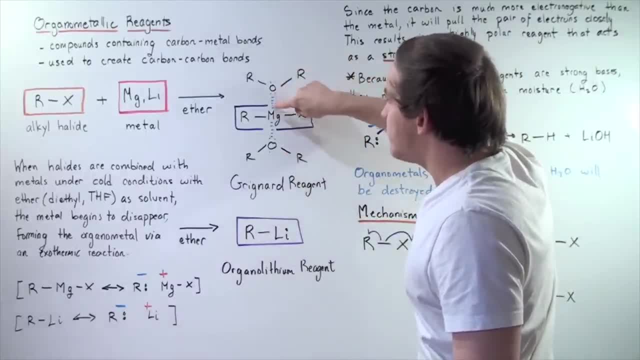 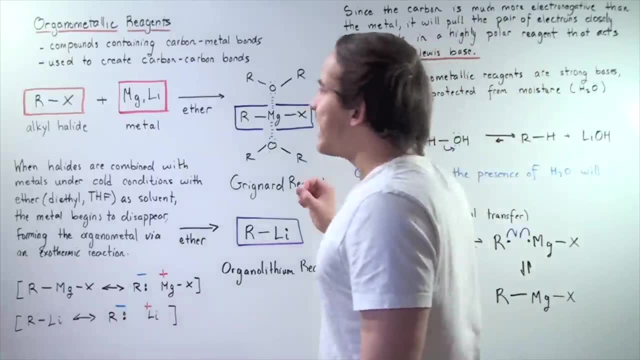 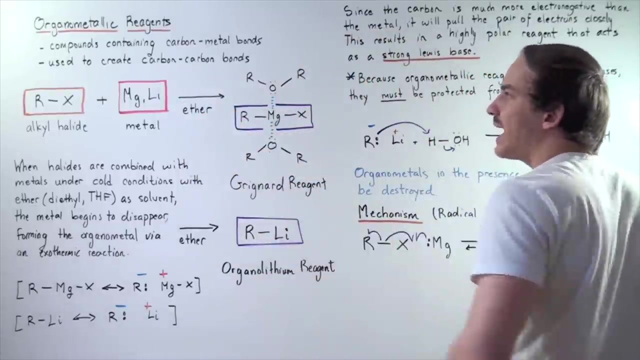 So these two ethers stabilize via the following induced polar bonds: polar intermolecular bonds. Now, What happens when lithium is mixed instead of magnesium? When lithium is mixed, the following organometallic reagent is produced, known as organolithium reagent. 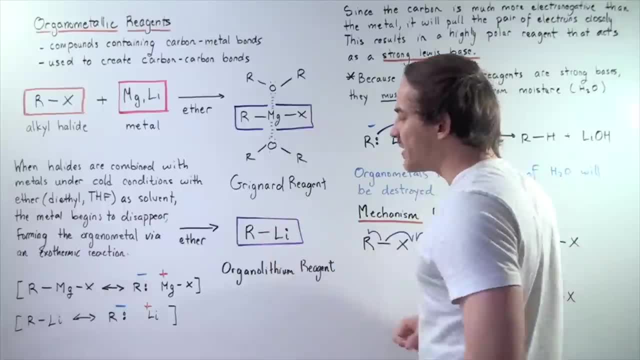 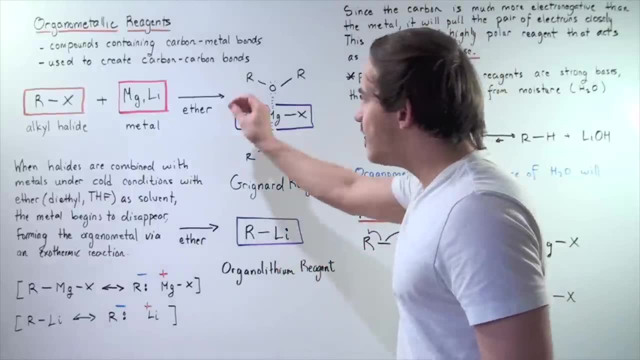 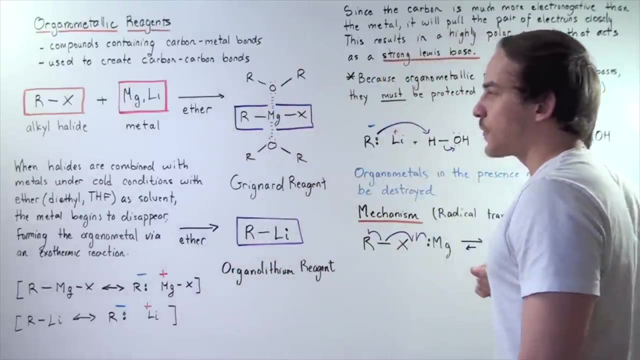 And here we simply have our R group attached to our lithium, So we have the covalent bond here. Now notice: in this case the ether does not stabilize our organometallic reagent the same way that it stabilizes lithium It stabilizes in the first case. 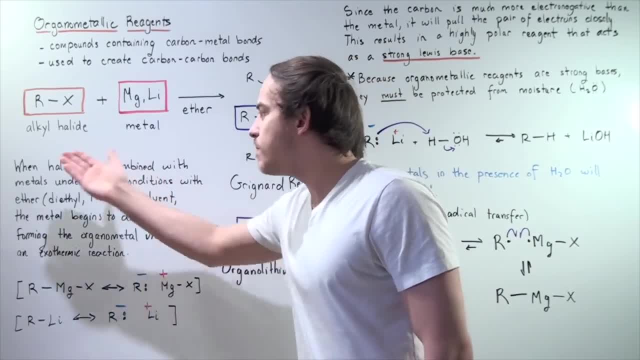 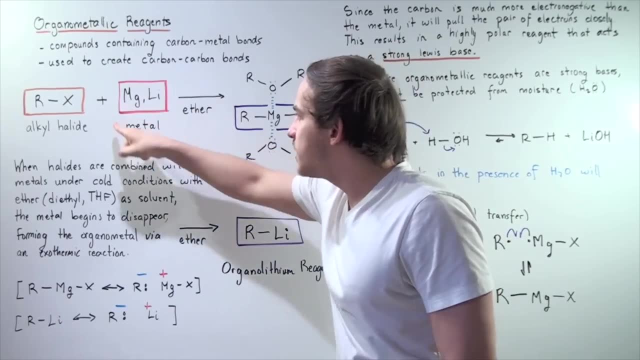 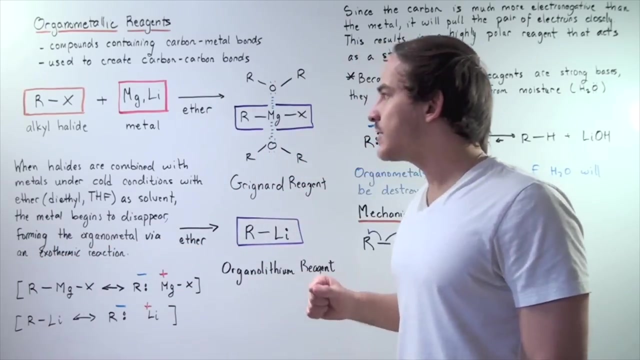 So, once again, when halides are combined with metals under cold conditions, with ether as solvent, the metal begins to disappear. So this begins to disappear, forming the organometallic reagent via an exothermic reaction. So this is an exothermic reaction. 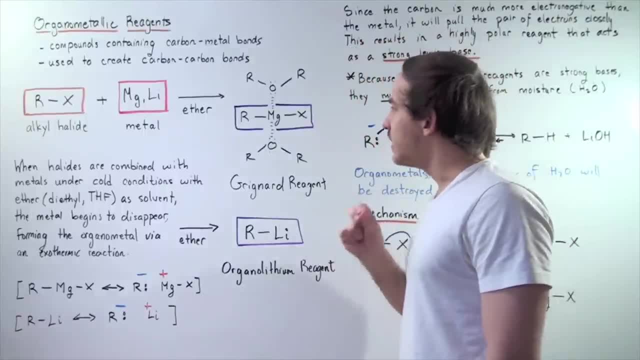 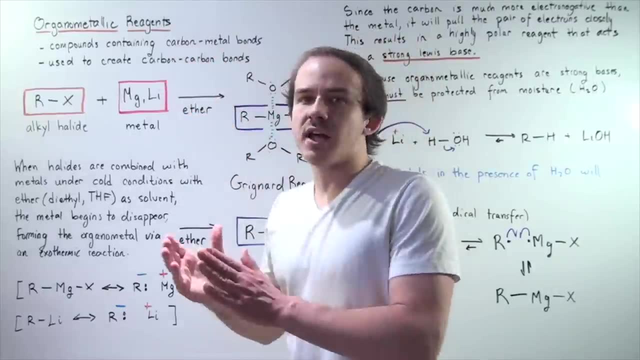 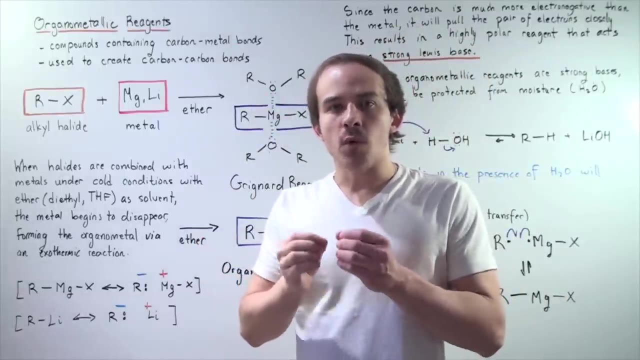 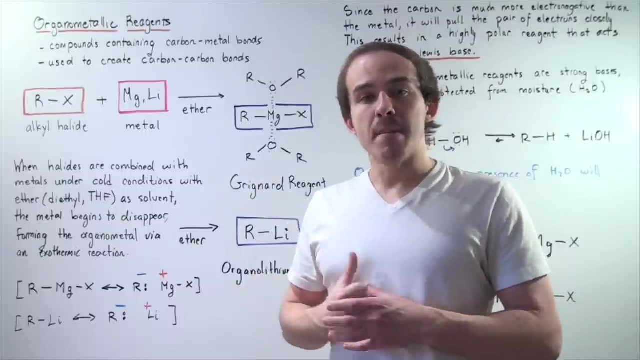 It releases energy. So Let's examine our carbon-metal bond. So what is a carbon-metal bond? Well, carbon is found on the left side of the periodic table. The metals are found on the right side. That means we're going to have a relatively electronegative atom, the carbon, and a not electronegative atom, the metal. 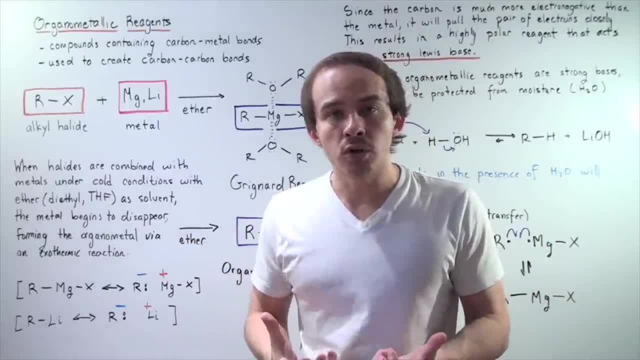 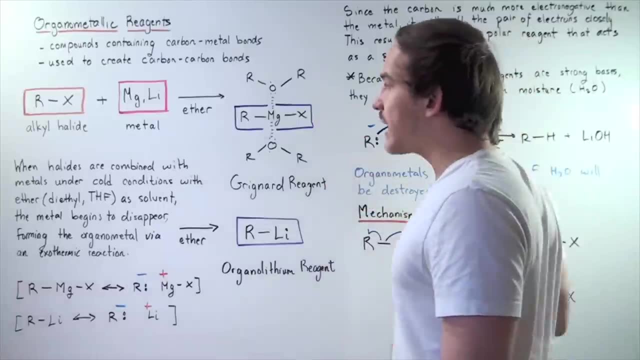 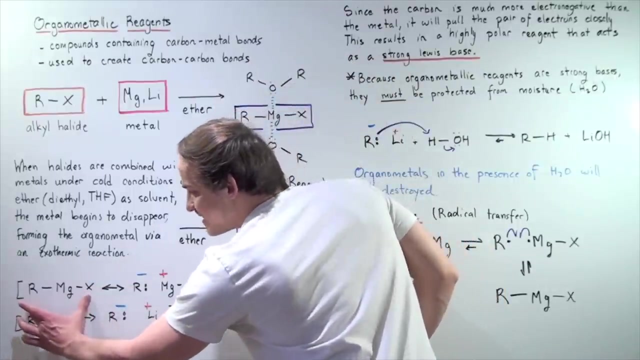 And that means these two bonds will be very polar. In fact, if we look at the resonance forms for these two organometallic reagents, we see the following happen: We see that one of the resonance forms is this and a second one is a form that has two electrons on the R. 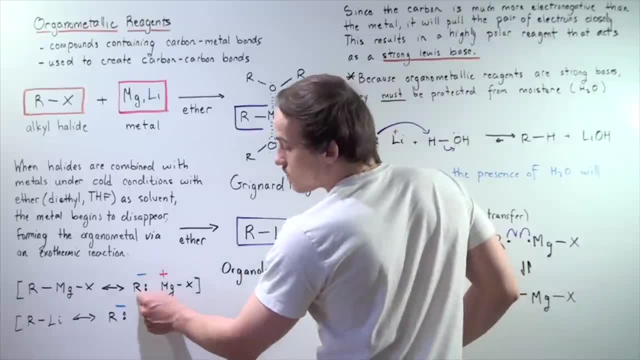 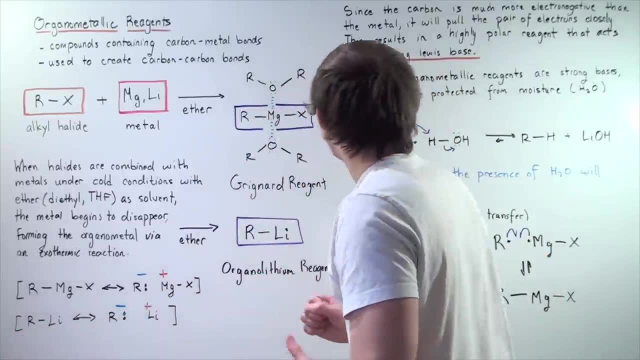 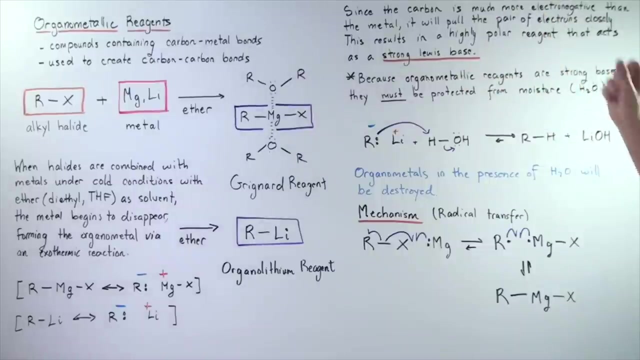 so this R has a negative charge and this magnesium, the metal, has a positive charge. Likewise the same for this case. So, once again, since the carbon is much more electronegative then the metal, it will pull the pair of electrons closely. 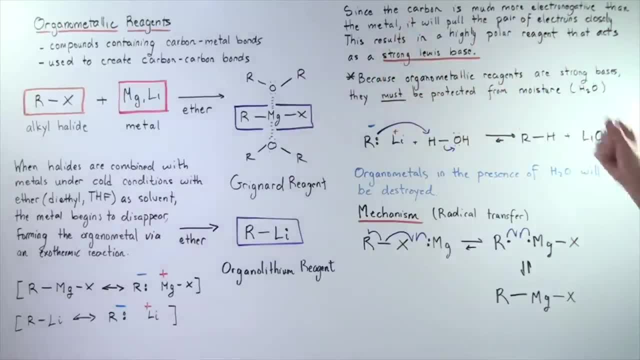 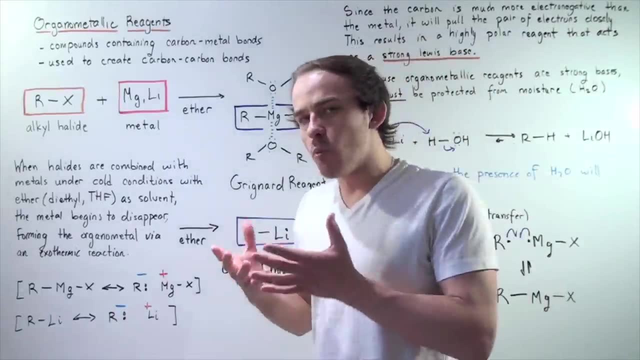 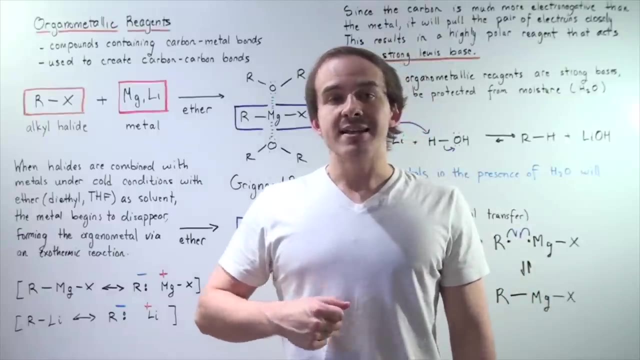 This results in a highly polar reagent that acts as a strong Lewis base. So, once again, because our carbon is so much more electronegative, it pulls those electrons more strongly than our metal does and, as a result, the electrons are found much closer to the carbon than to the metal atom. 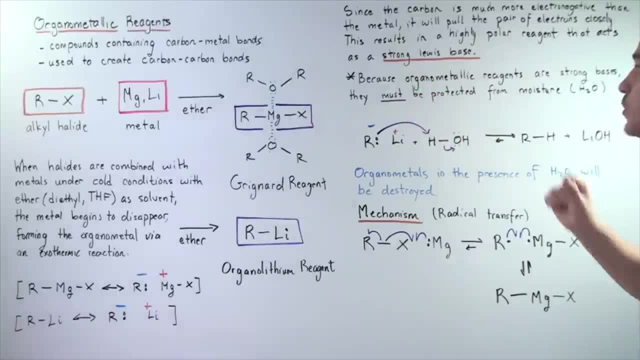 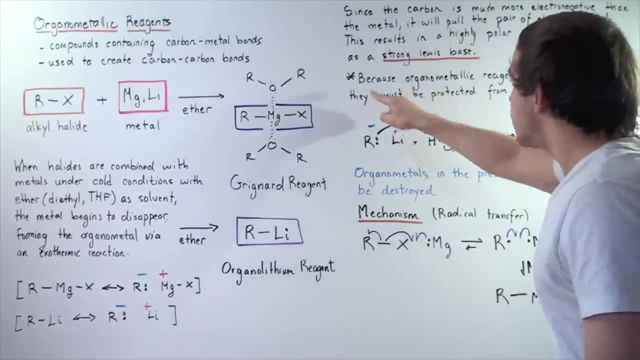 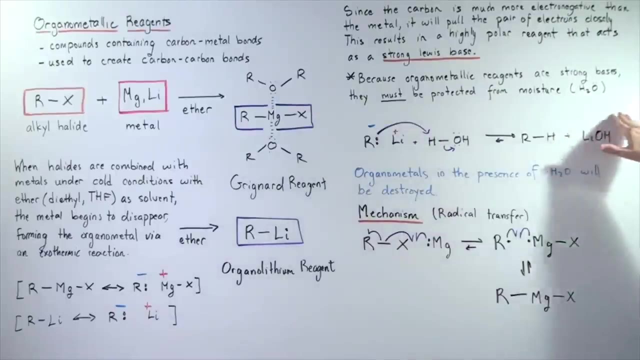 And this creates a strong Lewis base, Now a very important product of this result. Because organometallic reagents are strong bases, they must be protected from moisture. In other words, earlier I said that the solvent must be an ether. 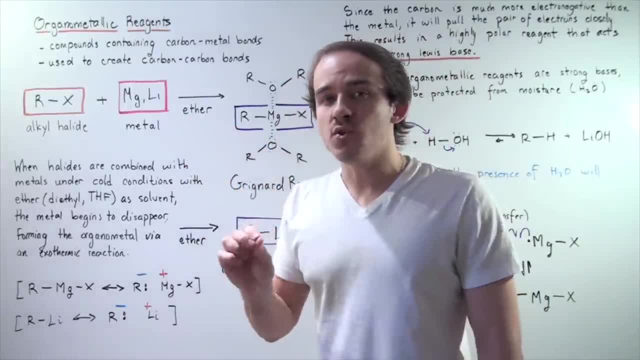 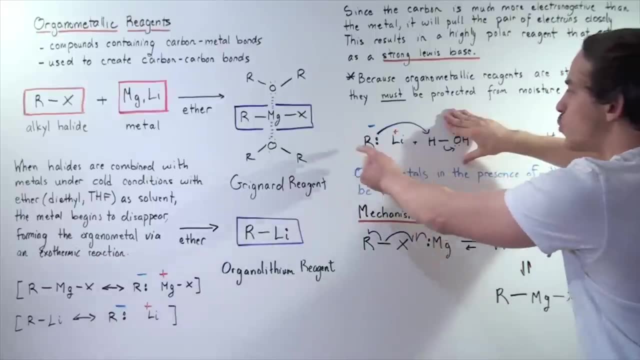 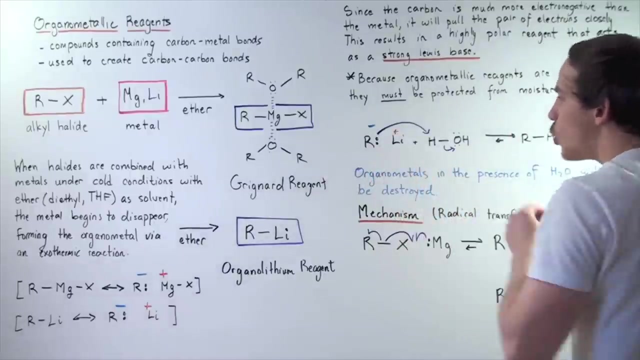 a nonpolar solvent. If we use a polar solvent, such as water, the water will react with the solvent, With our Lewis base, with our organometallic reagent, in the following manner. So this pair of electrons will take this H atom. 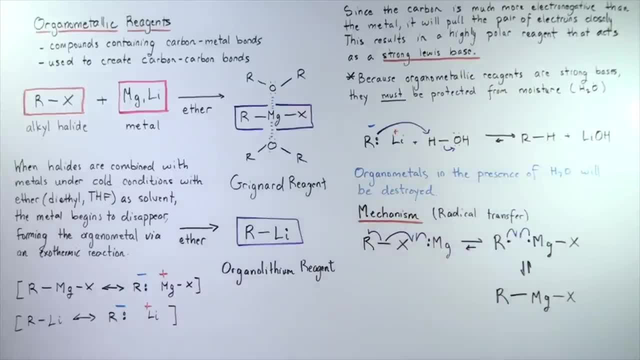 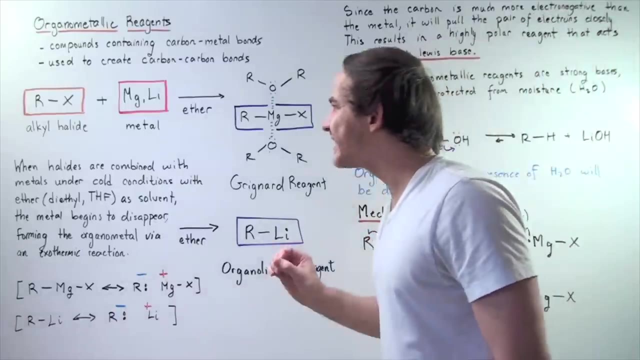 and will create this Rh, so a hydrocarbon And the lithium will combine with our hydroxide group. So important, important, important Organometalls in the presence of H2O will be destroyed. So it's important to protect. 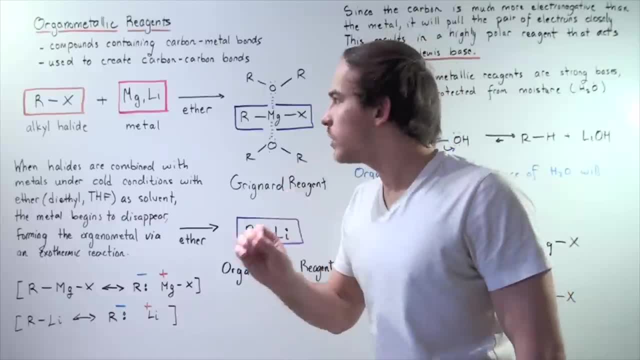 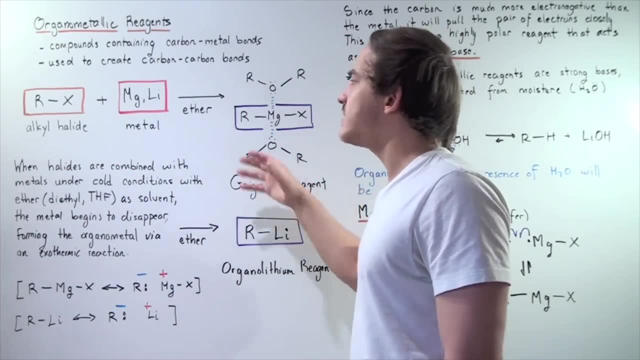 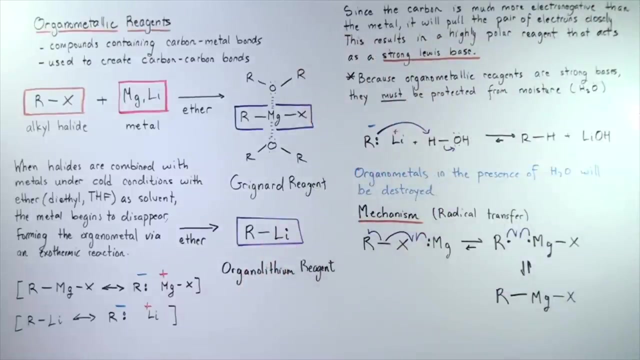 our reactants, from moisture, from polar compounds such as water. Now, so far we have discussed how this reaction takes place. but what is the mechanism? Well, the mechanism actually involves a radical transfer. In other words, one of the electrons breaks off and goes onto the R. 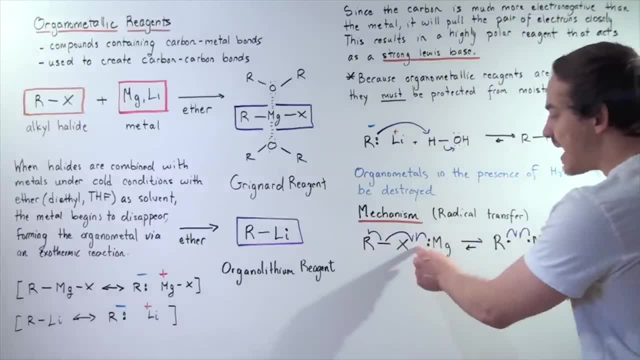 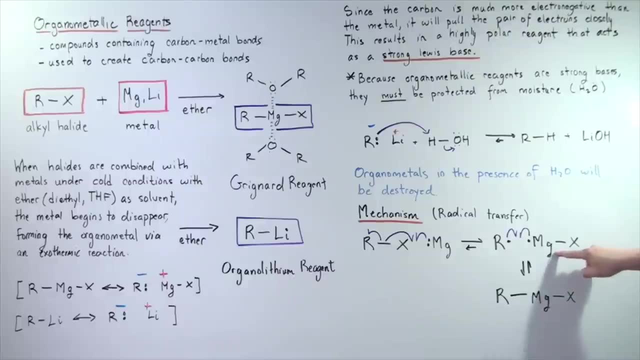 the second electron breaks off and goes onto the X and one of the electrons from magnesium combines to form a bond. So we have a covalent bond between magnesium and the halogen, and the magnesium has a spare electron, it has one electron. 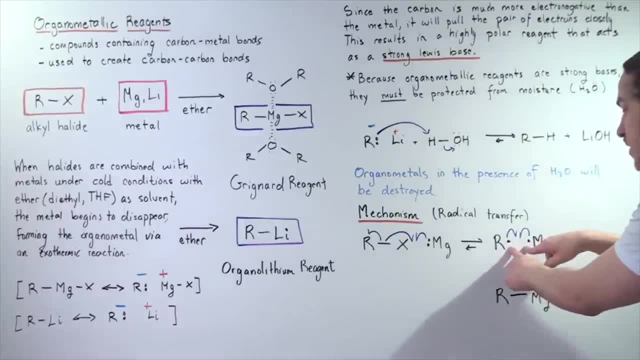 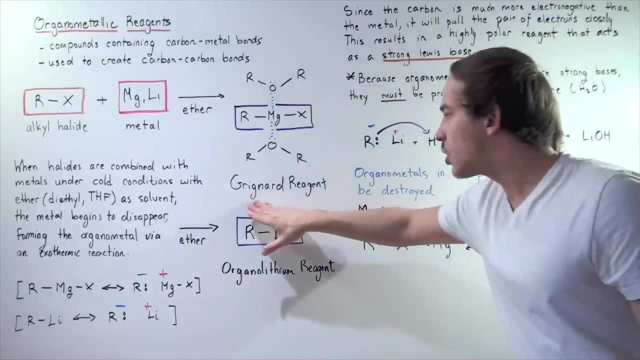 And now this electron combines with this electron to form our final product, the organometallic reagent, in this case the Grignard reagent.